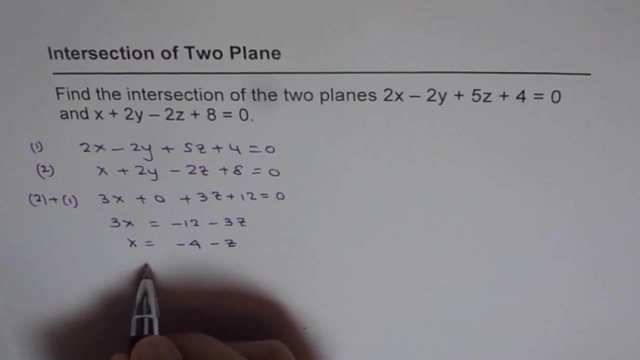 Now, if we assume z to be equals to a parameter, t, so let z equals to t. In that case, x is equals to minus 4 minus t. So that is how you know: we introduce parameters and we get a solution in terms of a parameter which will result into a line. So remember one thing: that we are solving two equations and we have three variables, So we can't really solve it right. So we'll have to use parameters to solve this particular equation. 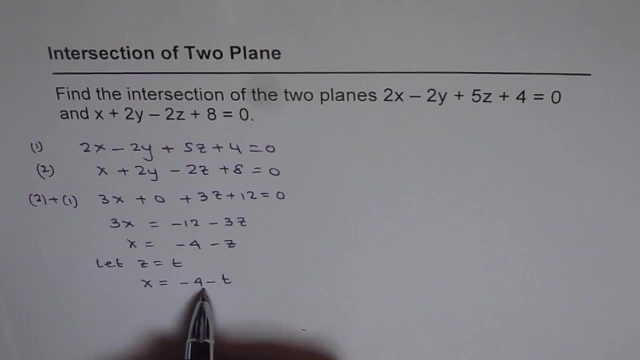 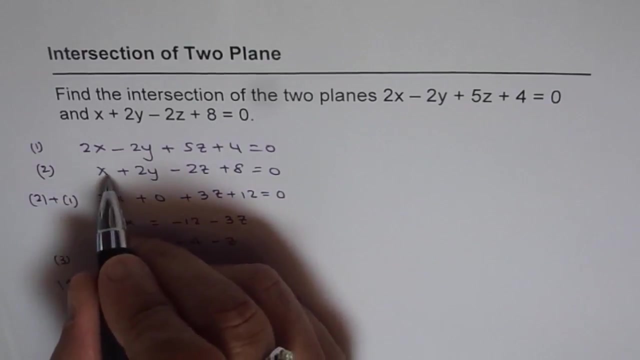 Now we know z is t, x is minus 4 minus t. So we'll use these two in one of our equations. So we have- let me call this- three and four as the z and x values. So we'll substitute those values in equation 2 and then solve for y. So we have x. so instead of x I'll write minus 4 minus t. So let me write equation 2 first here. 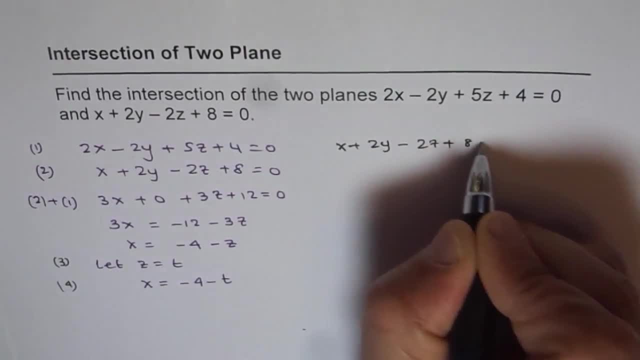 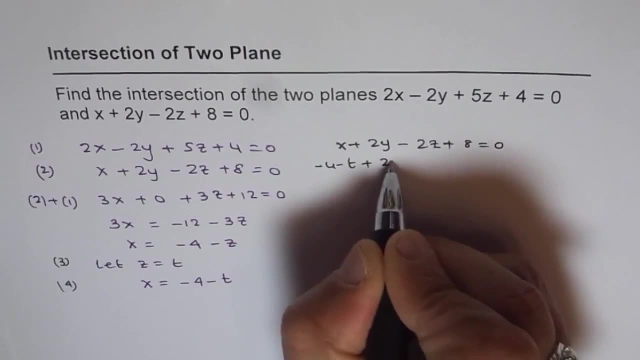 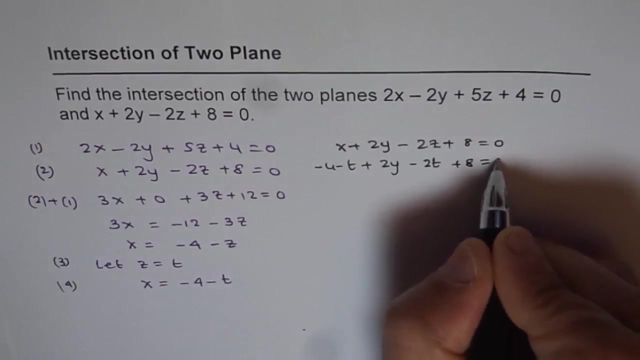 2y minus 2z plus 8 equals to 0, and now instead of x I'll write minus 4, minus t plus 2y, and instead of z we have 2t, the parameter defined here- plus 8 equals to 0. and now we can solve for y in terms: 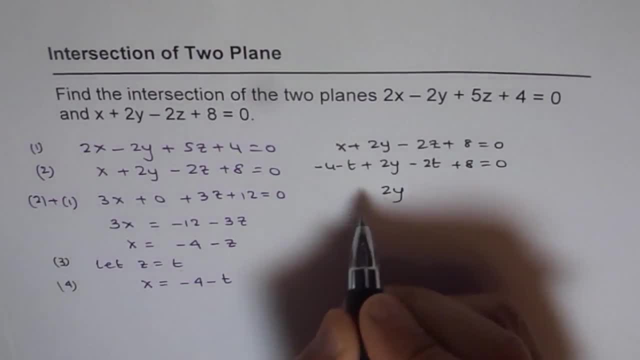 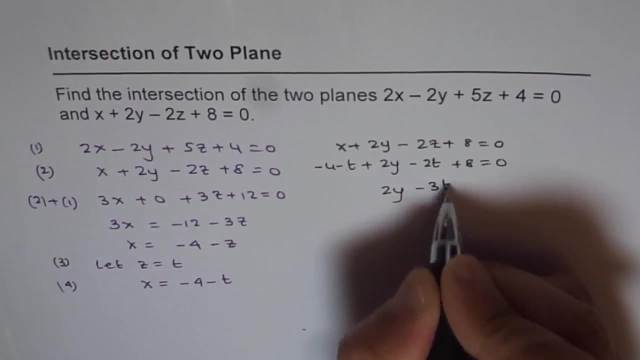 of t, right. so we have 2y here, 2y, and as far as t is concerned, minus 1 and minus 2 gives us minus 3t. as far as the constants are concerned, minus 4 and plus 8 gives us plus 4 equals to 0. 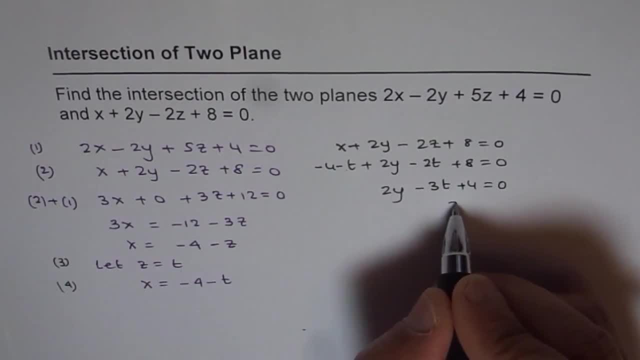 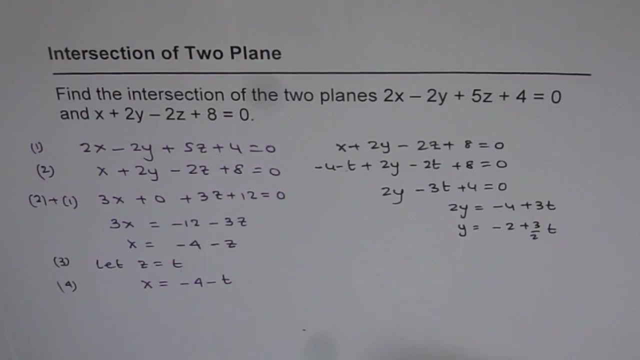 so from here we can write: 2y equals to minus 4 plus 3t, or y equals 2 divided by 2. we get minus 2 plus 3 over 2t, right, so we get a solution here, and that is the equation of a line. 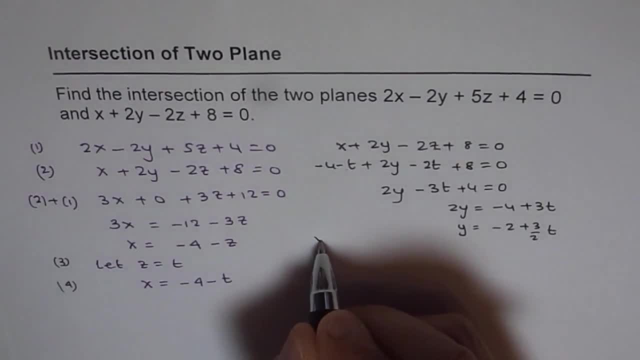 and then the line is: x equals to minus 4 minus t, y is equals to minus 2, 3 over 2 plus 3 over 2t and z equals to t right. so that is the equation of the line which gives us a solution for this particular.